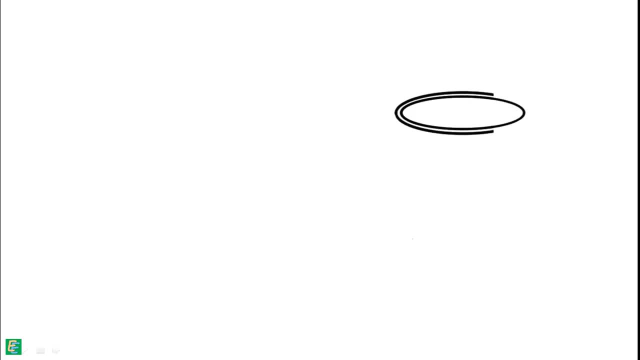 constant head permeameter. This instrument consists of a cylindrical mould which is connected with two manometers at its curved surface. First we measure its internal diameter and determine its internal area, which we will use to measure the permeability of the soil. We say capital A. This mould is attached with two filter discs at the top and the bottom. 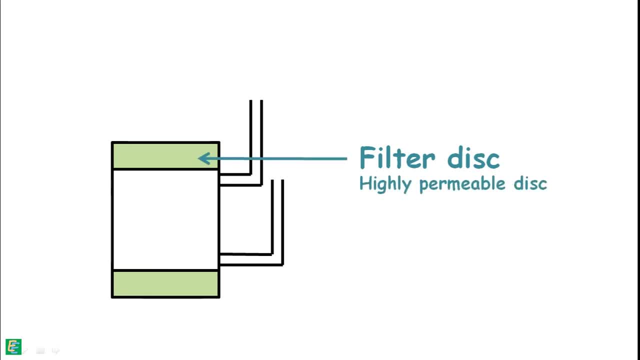 These discs are porous and highly permeable. These are also provided with inlet and outlet facilities. We can perform this experiment for both disturbed and undisturbed soil sample. We fill the mould with our sample soil and compact it to a density which may be the representative. 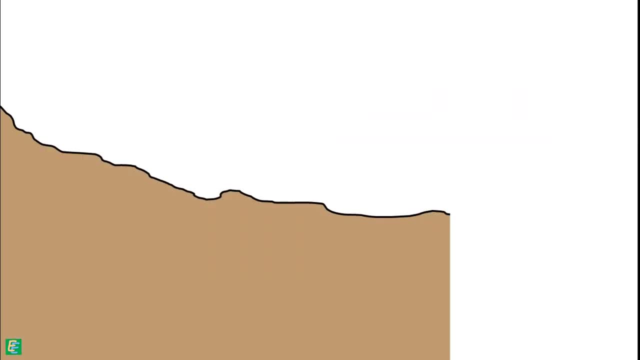 of the field conditions Or for an undisturbed sample. we take out the soil sample from the ground and trim it to the dimensions similar to that of the mould. We place the sample inside the mould between the porous discs. Some space will be left between mould and specimen that we will fill. 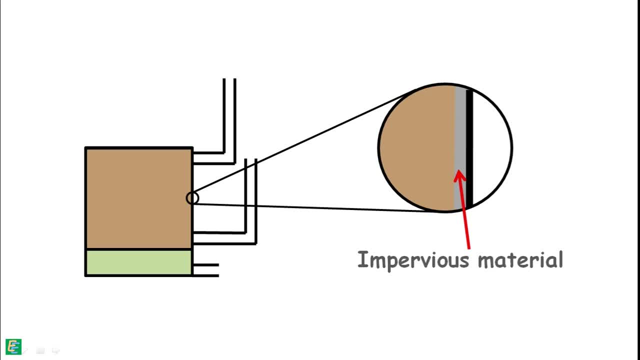 with some impervious material such as cement slurry. The inlet of the instrument is then connected with a constant head water reservoir and water is released into the soil sample. When water flows through the soil, water level in the reservoir tend to decrease fast because 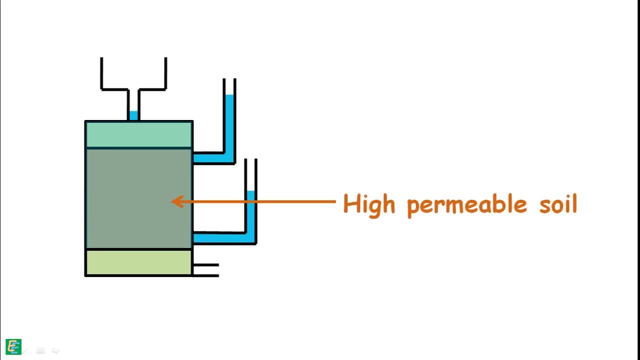 soil we took is highly permeable soil, so high amount of water will flow through it. But with the proper arrangement, the water level in the reservoir must be kept constant. Before beginning the experiment, we first let the soil sample get fully saturated and 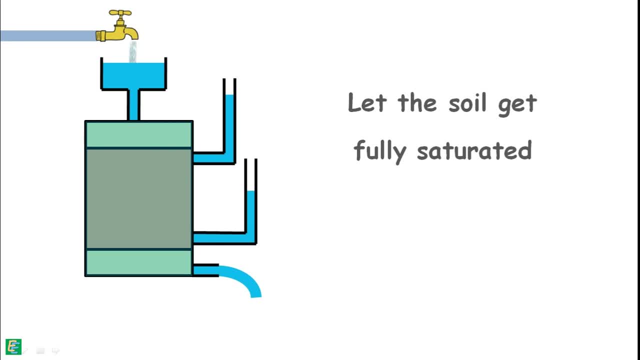 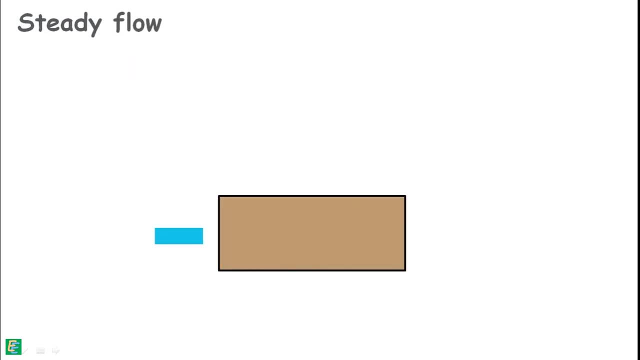 even after that, we allow the water to flow out for some time so that a steady flow can be attained. A steady flow is the one in which the quantity of liquid flowing per second through any section is constant. We will also notice that after the water has been released into the soil, the water level 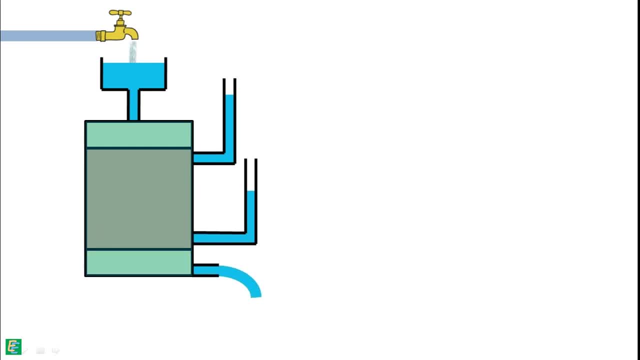 in the manometers has risen up. The height of the water column in the manometer shows the total head or total energy of the water in the soil sample at this level. The difference of the heights of the water level in these two manometers is the difference. 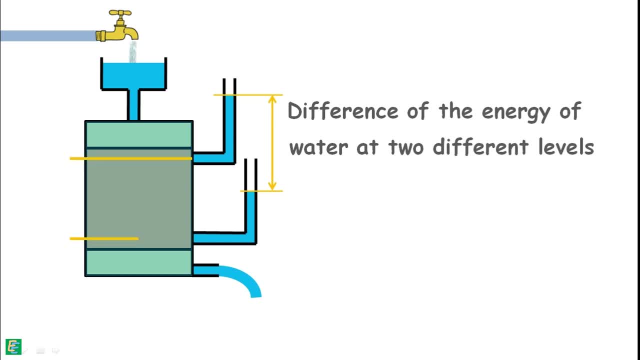 of the total energy of the water at these two levels in the soil sample. This difference of energy of the water drives it to flow in the soil from one point of high energy to the other, to the point of low energy. we note down the difference of the heads of these. 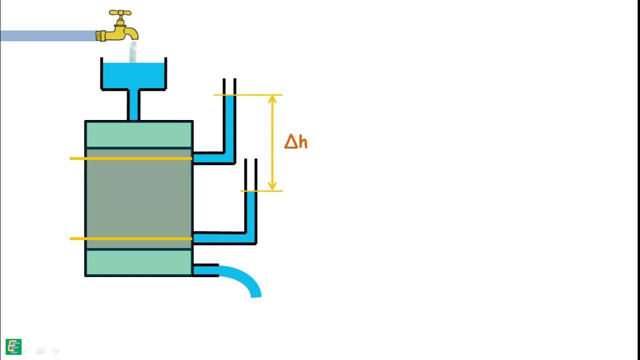 manometers as Delta H, and also note down the distance between the points in the soil where these heads for, measured by these manometers as L. we wish to maintain this difference of heads in the manometers so that we can maintain the hydraulic gradient inside the soil by keeping the head of the water reservoir. 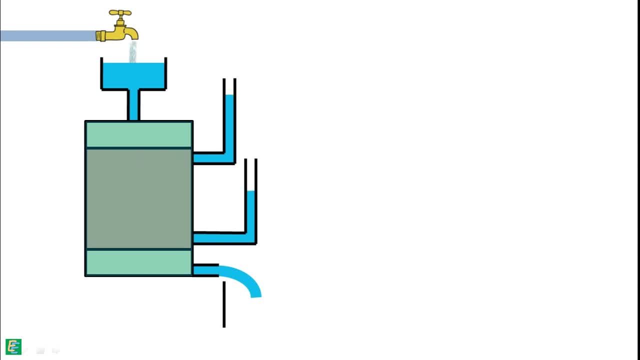 constant. we place a graduated jar at the outlet to collect the water coming out of the sample and a stopwatch is started. we collect the water in the jar for a fixed time interval, T, and note down the amount of water collected as capital Q. now for this system we may apply Darcy's law, which state that the velocity of 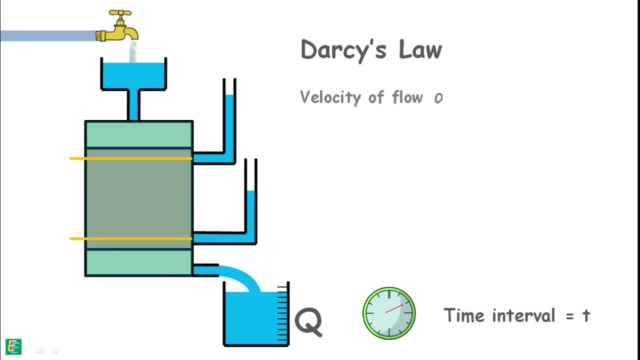 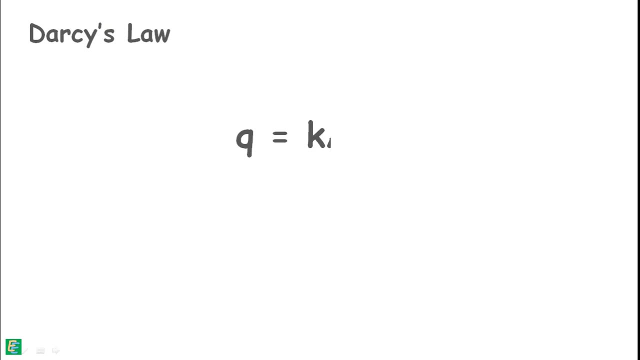 flow of liquid between two points in the soil is directly proportional to the hydraulic gradient of the water applied to it, and K is added as proportionality constant, which is called coefficient of permeability of soil. we also write the law for discharge as this: I is the hydraulic gradient and can be written as this here discharge can be. 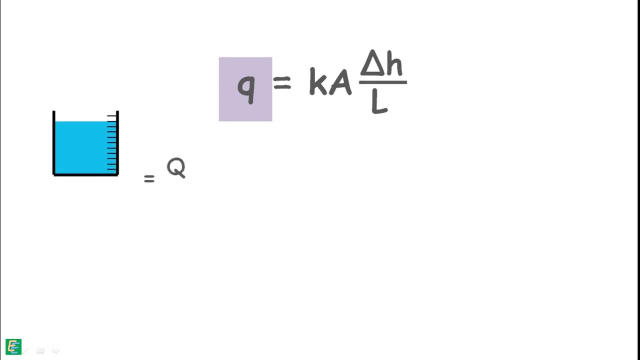 calculated as the volume of water collected, capital Q divided by the time interval T. we have calculated the area of mould, capital A. we have also determined the head difference and the length L over which the head changed. so we have measured all the required values in this equation to calculate and know the permeability of the soil sample. 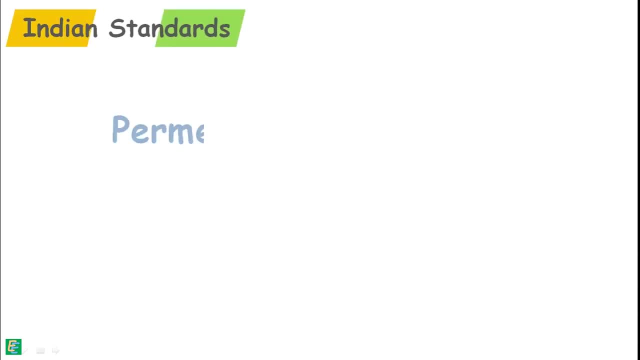 according to the Indian standards, we report the permeability values at 27 degrees Celsius temperature. so if we measure the temperature of the water as 3 degrees Celsius, then using this equation we get we can find the temperature of water as T degree Celsius. then using that theấ� 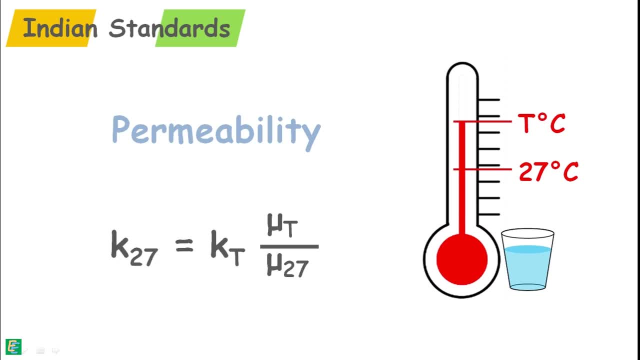 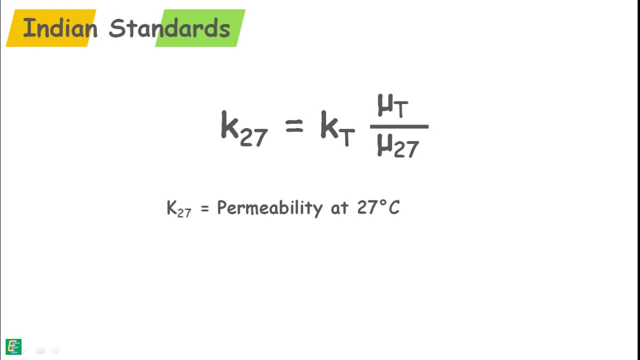 Using this formula we can calculate the permeability at 27 degree Celsius. Here, K27 is the permeability of the soil at 27 degree Celsius. KT is the permeability of the soil at test temperature. T- MuT is the coefficient of viscosity at test temperature.